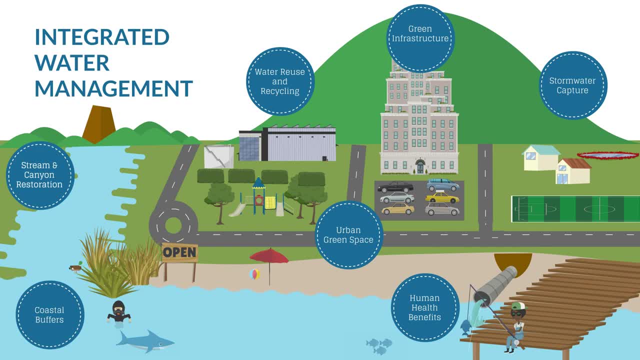 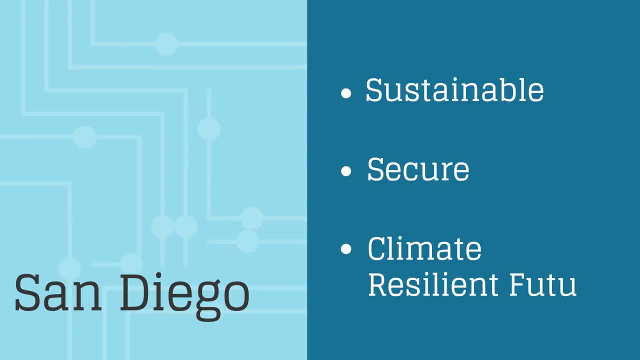 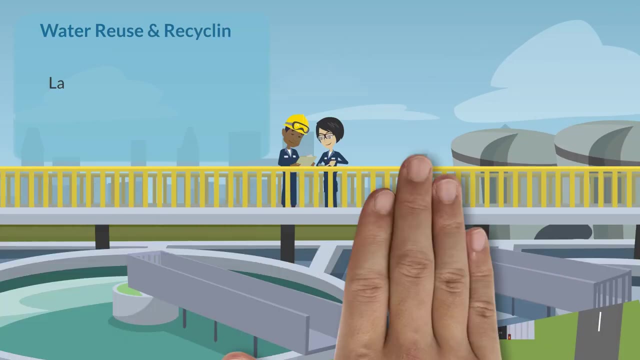 water supply reliability, climate change mitigation and the health of humans and wildlife alike. Adopting these practices has the power to put San Diego on the path toward a more sustainable, secure and climate resilient future. Let's explore Large-scale water. recycling provides reliable, locally sourced drinking water while reducing 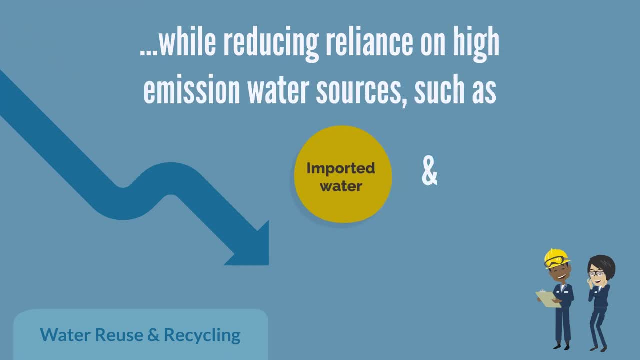 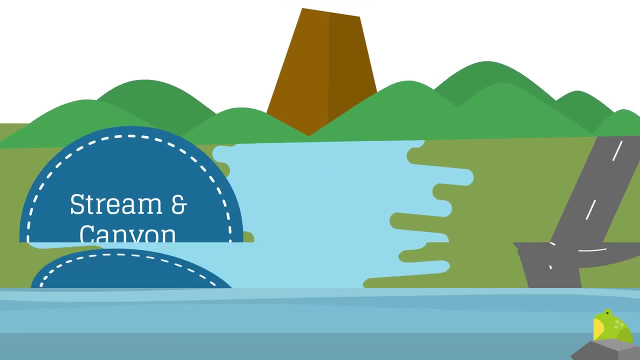 reliance on emission-intensive water sources such as imported water and seawater. desalination, Removal of concrete channels and the restoration of water supply systems is an important part of the process. In addition, the restoration of natural stream systems creates habitat for wildlife sequesters carbon. 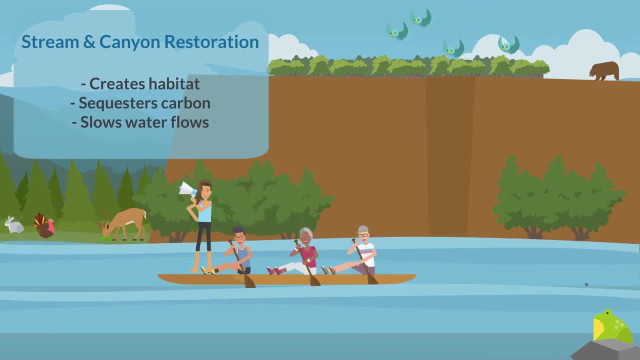 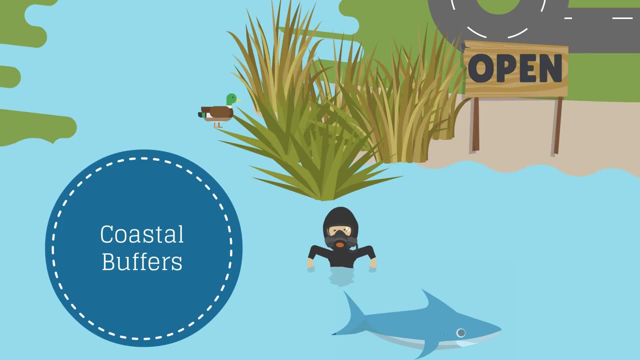 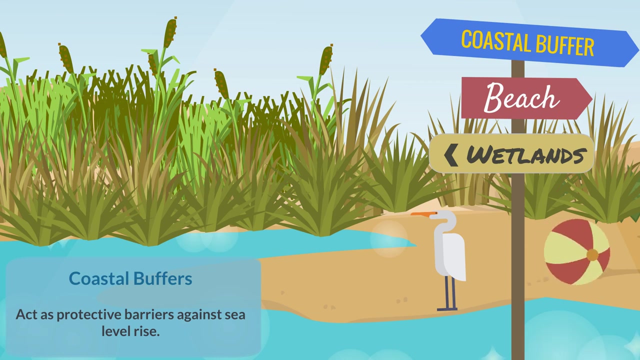 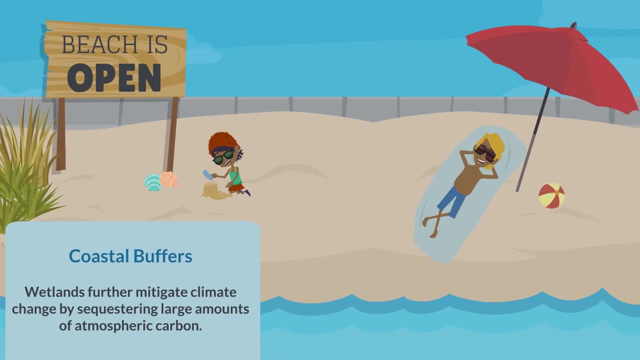 and slows water flows, which reduces erosion and allows for natural filtration of pollutants from water. Restored coastal wetlands and protective bluffs created by natural sediment deposition as the result of stream restoration act as protective barriers against sea level rise. Wetlands further mitigate climate change by sequestering large amounts of atmospheric carbon. 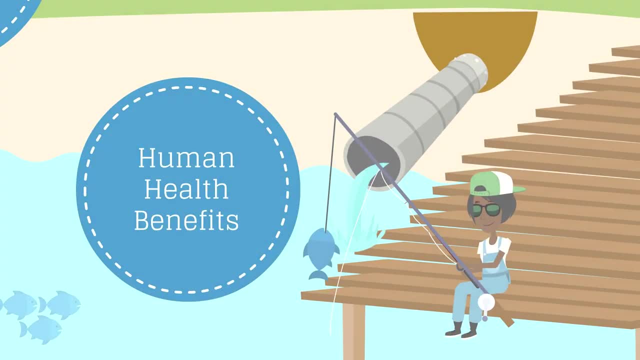 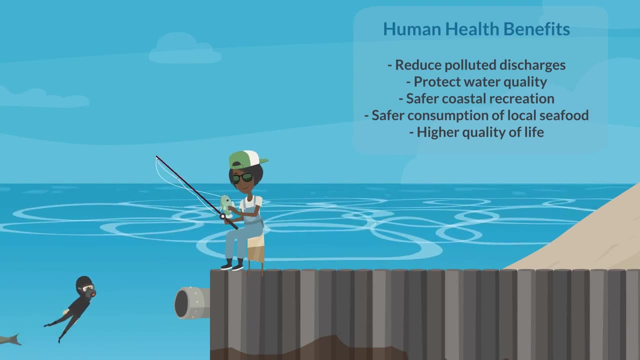 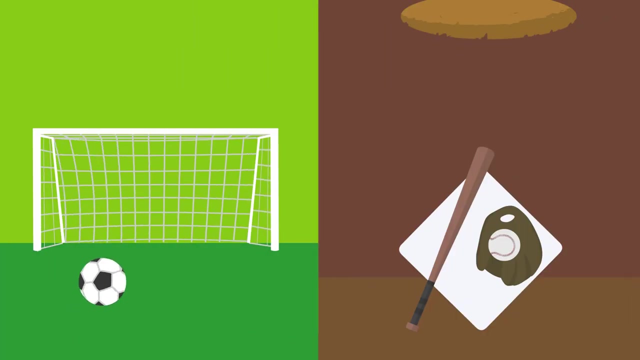 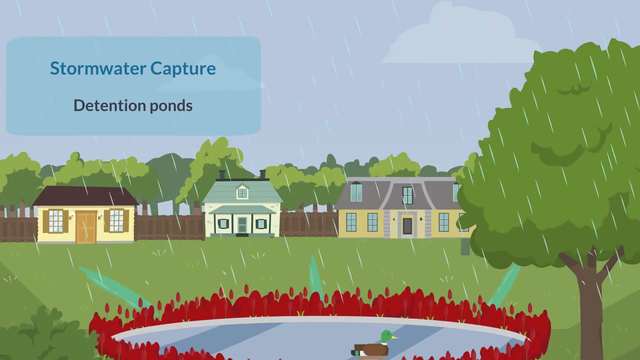 Integrated water management practices reduce polluted discharges and protect water quality. This makes for safer coastal recreation, safer consumption of local seafood and higher quality of life. Small and large-scale stormwater capture from retention vaults beneath parks to detention ponds in community garden space reduce polluted discharges and protect against. 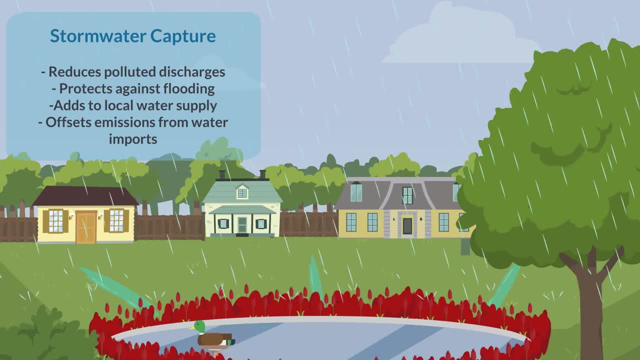 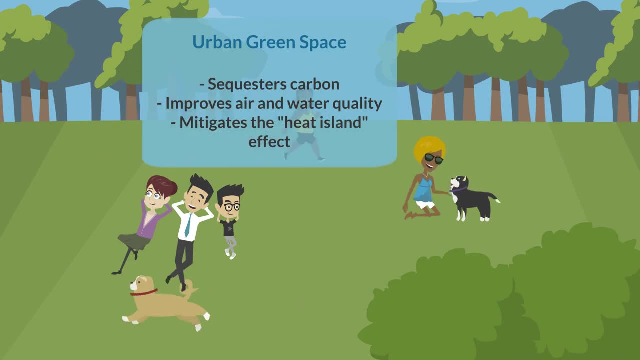 flooding while adding to local water quality. Restored coastal wetlands and protective bluffs add to local water supply and offsetting emissions from water imports. Parkland, incorporated into commercial, residential and community spaces, sequesters carbon, improves air and water quality, mitigates the heat island effect and provides community health. 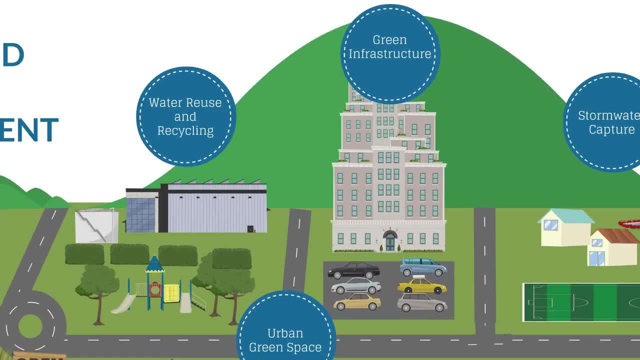 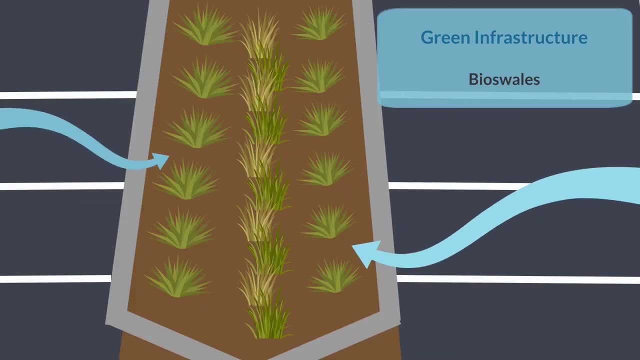 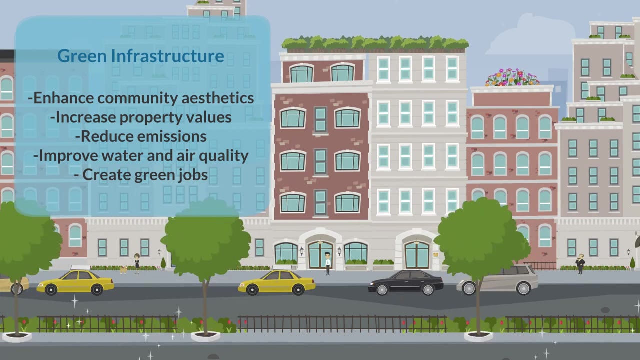 benefits. The use of green infrastructure such as green roofs, permeable surfaces, community green space, bioswales and climate smart landscaping enhance community aesthetics, increase property values, reduce emissions, improve water quality and air quality and create green jobs. 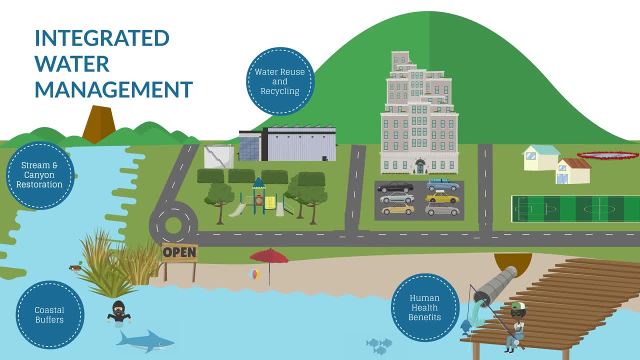 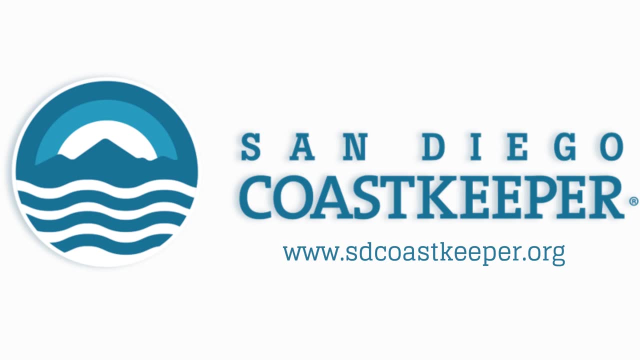 We hope you have enjoyed this introduction to the elements and benefits of integrated water management. To learn more, contact San Diego Coastkeeper at wwwsdcoastkeeperorg.